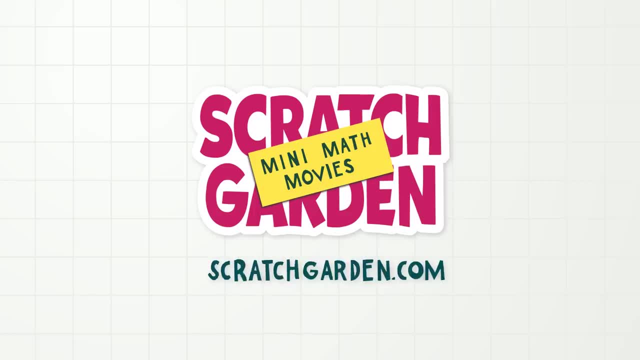 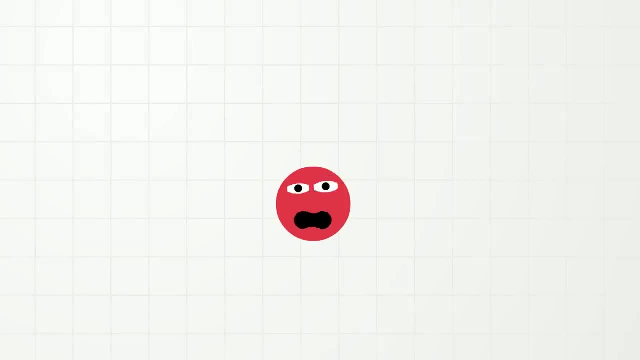 Oh hi everybody! Today I am going to talk to you about numbers. And adding and subtracting numbers. And maybe even donuts. I really like donuts. So, we all know that numbers can be joined together to make bigger numbers. We call this adding. Adding! And we also know that we can take away numbers from bigger numbers to make smaller numbers. We call this subtracting. Subtracting! Let us use an example. We need a volunteer. How about… Sloth! It's a sloth! Okay, here is a sloth. And we see that sloth has two donuts. One, two. What happens if we add one, two, three more donuts? Yes, that's right, sloth gets happier! But also, mathematically, if we add two and three together, we get five. Five donuts! Now what happens if we subtract? One, two, three, four donuts from sloth. Yes, that's right, sloth gets sadder. But also, mathematically, if we have five and we subtract four, we only have one left. One donut! Wow, you did such a good job adding and subtracting, it's now playtime! Okay, that's enough. So, we can add and subtract. 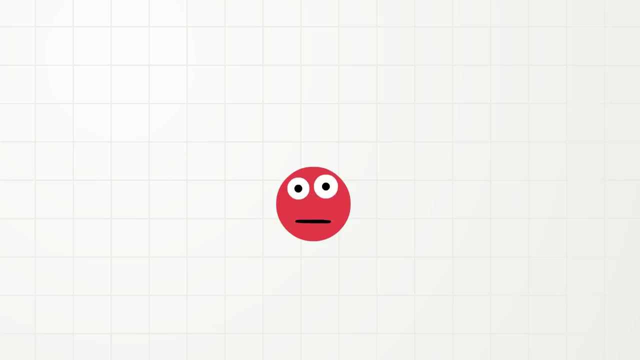 We can add and subtract with donuts, but did you know that we can also add and subtract with writing? No, it's true! We can do it by writing the numbers, or numerals, and also 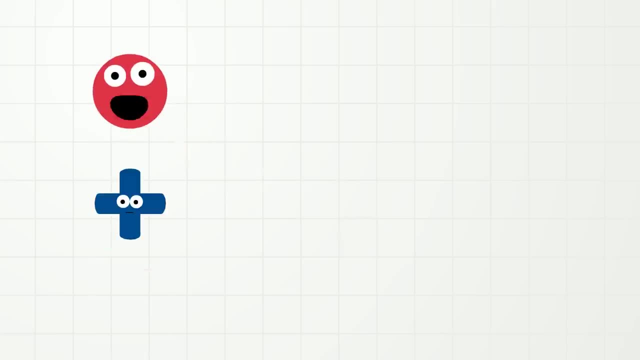 by writing with signs! This is a plus sign. This is a minus sign. And this is an equals sign. 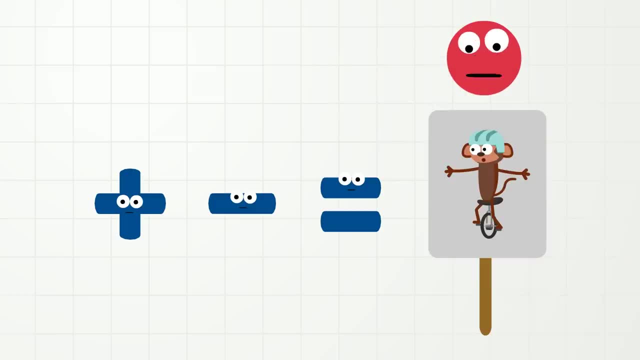 And this is a monkey riding instrument. a unicycle sign, but we never use that one in math. Please go away monkey riding a unicycle sign. 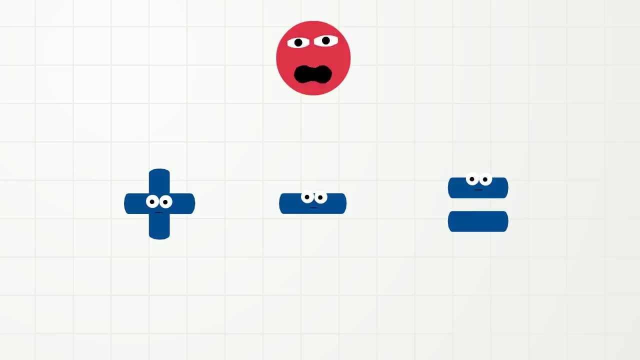 Ok great! So let's add and subtract the same number of donuts with sloth, but this time also write the numbers and the signs. Ready? Of course you are! Sloth, sloth. Finally. 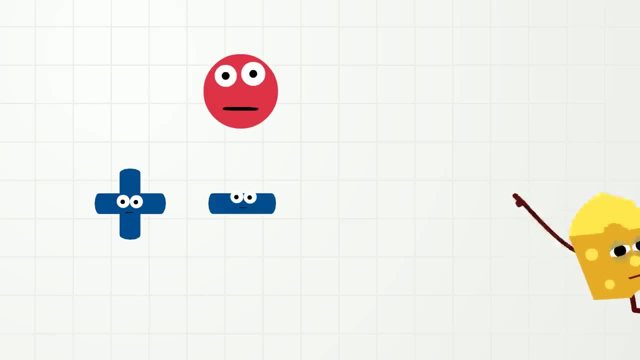 Is this plus or minus Accurate? And then, what about this? It's positive one. You read it, I read it. This is a positive sign, a unicycle sign, but we never used that one in math. Please go away, monkey, riding a unicycle sign. 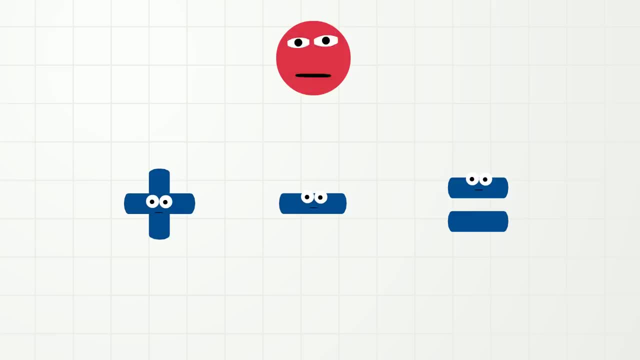 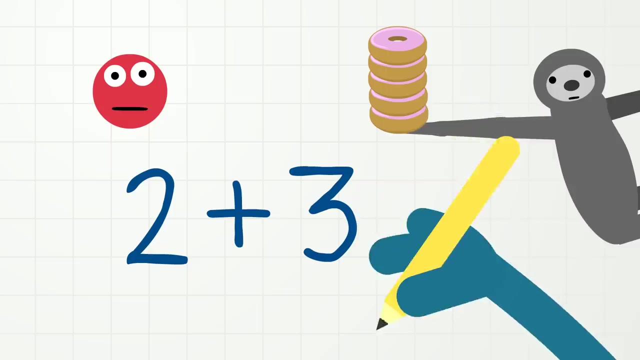 Ok, great. So let's add and subtract the same number of doughnuts with sloth, but this time also write the numbers and the signs. Ready, Of course you are Sloth, sloth. Finally, First, the adding Two doughnuts plus three doughnuts equals five doughnuts. 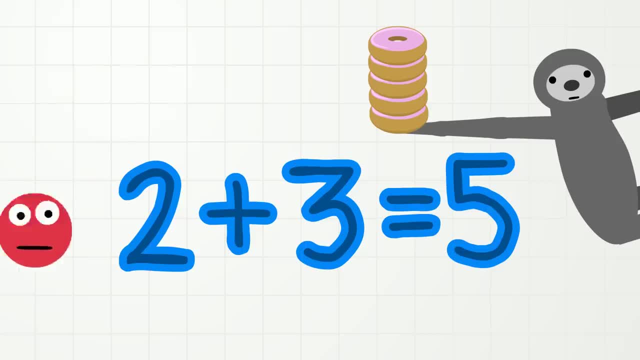 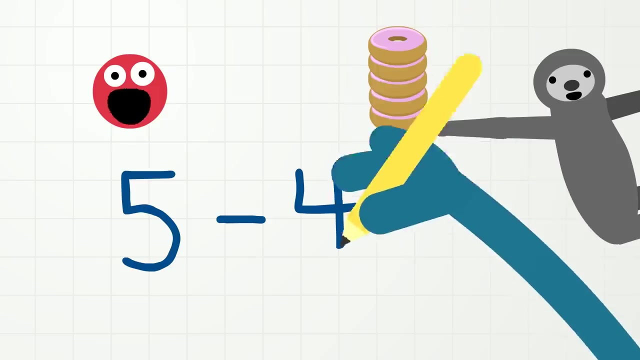 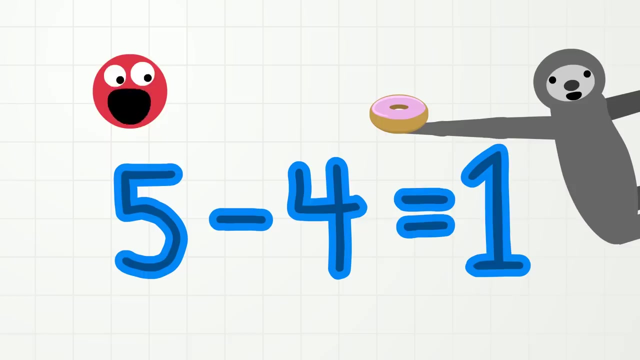 Two plus three equals five. Two plus sign three equals sign five. Happy sloth. Now, subtracting Five doughnuts minus four doughnuts equals one doughnut. Five minus four equals five. Five minus sign four equals sign one. Sad sloth. 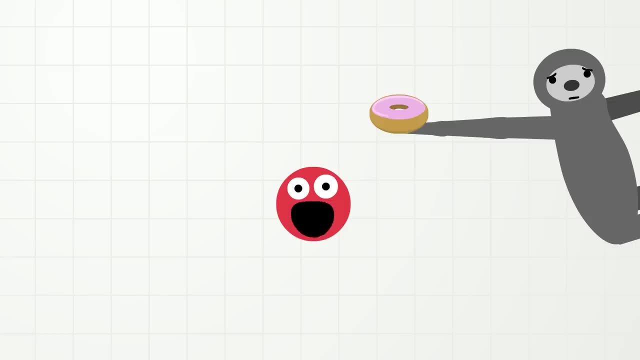 Ok, let's do another one, but with some different numbers and different doughnuts, Oh, purple. So let's see, We have one, two, three, four doughnuts And we add one, two, three, four doughnuts. 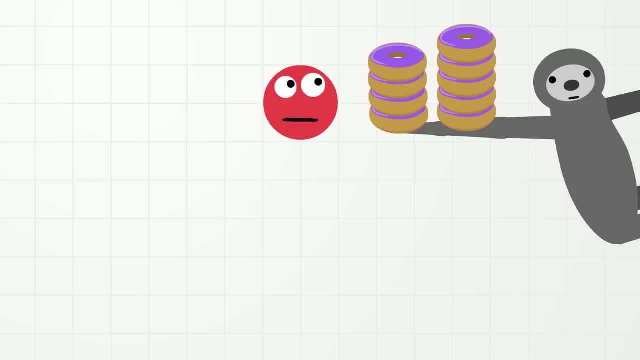 One, two, three, four doughnuts. One, two, three, four doughnuts. One, two, three, four, five doughnuts. So we have anybody know That's right. Nine doughnuts, Four plus five, equals nine. 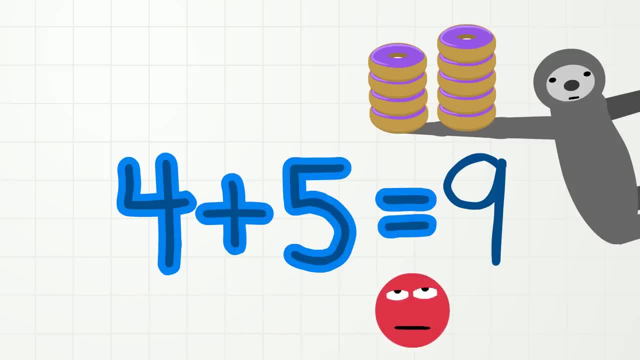 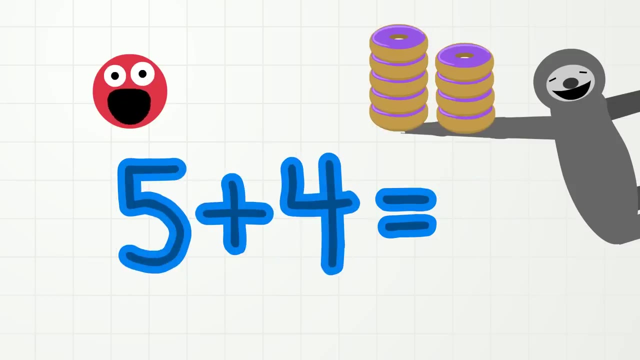 Four plus sign five equals sign nine: Super happy sloth. So I have a question: What do you think happens if we switch the four and the five like this: Now, how many doughnuts do we have? we have, That's right, the same number of doughnuts: 9 doughnuts. So 4 plus 5 equals. 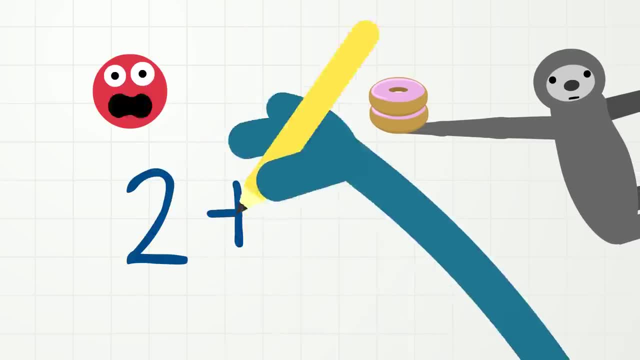 First, the adding. Two donuts plus three donuts equals five donuts. Two plus sign three equals sign five. 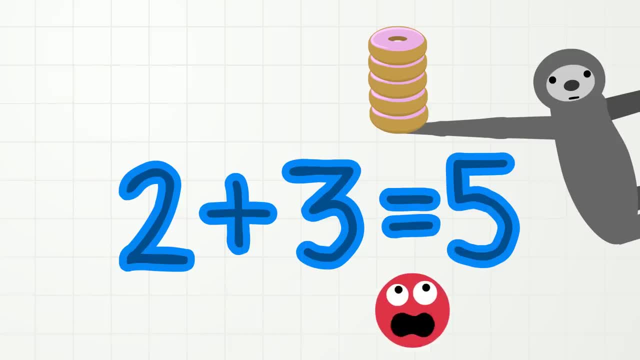 Two plus three equals five. Happy sloth! 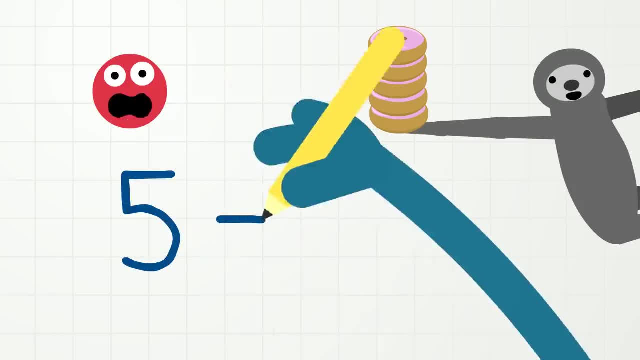 Now subtracting. Five donuts minus four donuts equals one donut. Five minus four equals five. 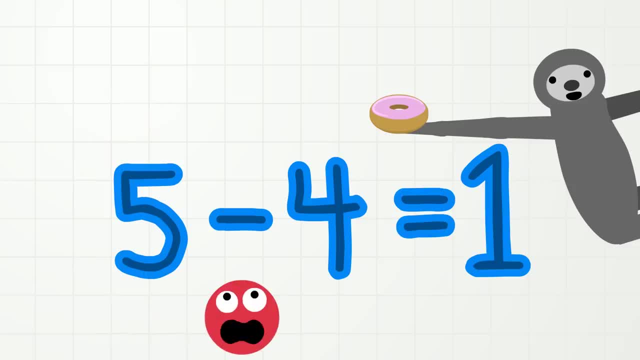 Five minus sign four equals sign one. Sad sloth. 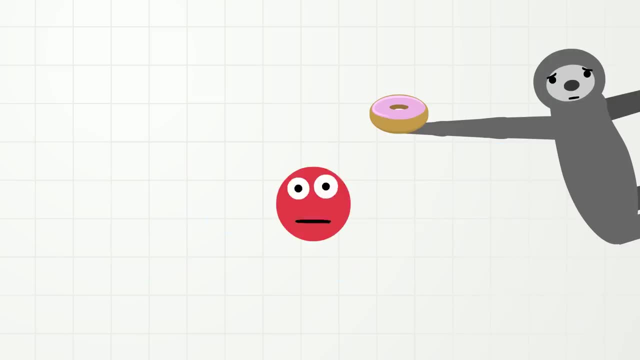 Ok, let's do another one, but with some different numbers and different donuts. 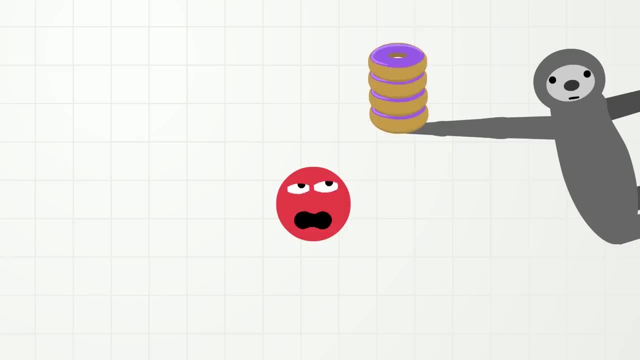 Oh, purple. So let's see. 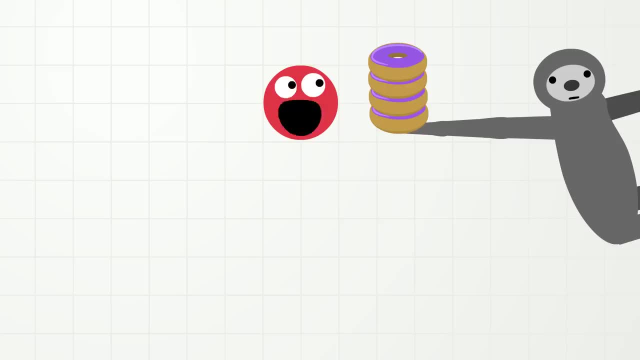 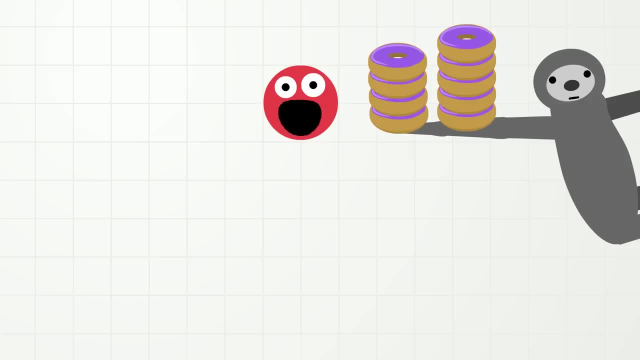 Five donuts. So we have... Anybody know? That's right! 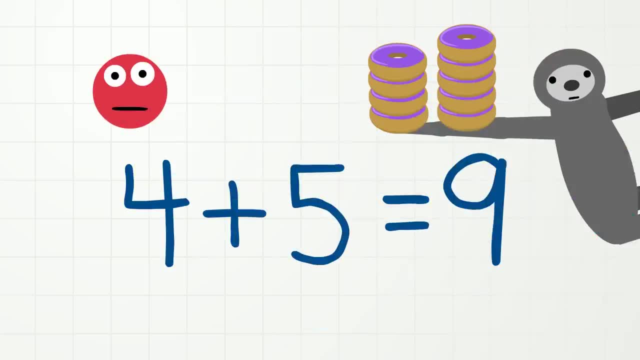 9 donuts. Four plus 5 equals 9. 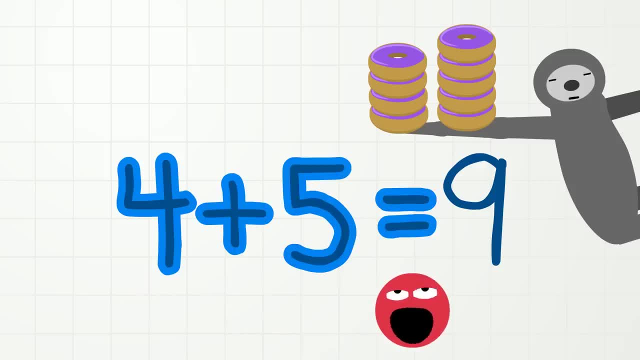 Four plus sign 5 equals sign 9. 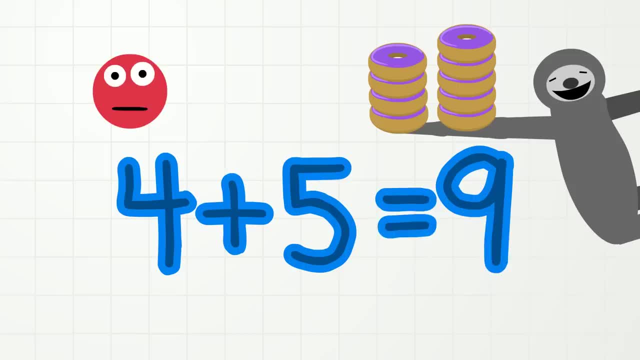 Super happy sloth! So I have a question. 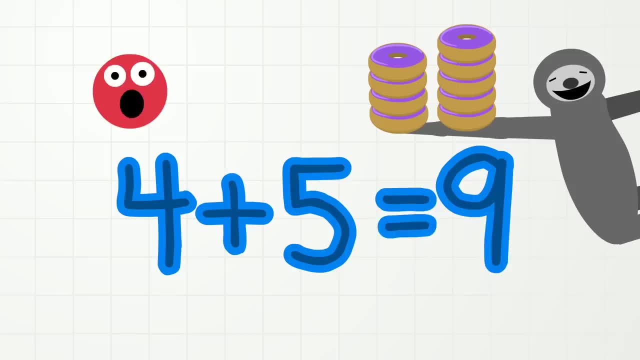 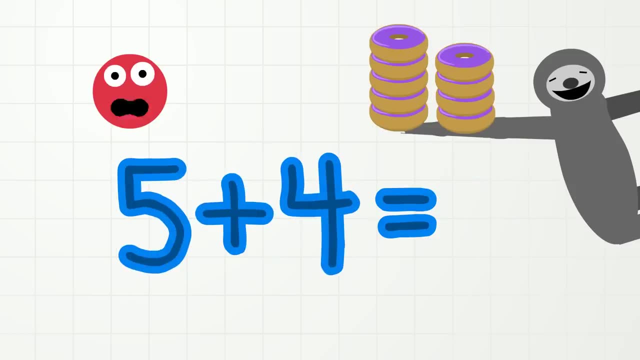 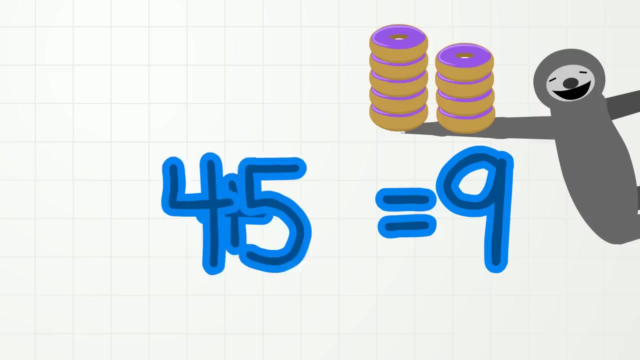 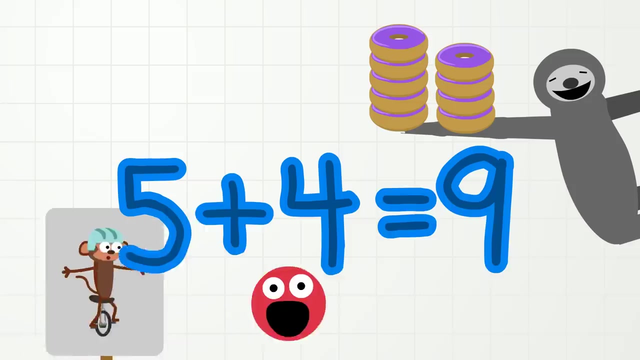 What do you think happens if we switch the 4 and the 5 like this? Now how many donuts do we have? One! One! Two! C mint! Swoosh! we have? That's right, the same number of doughnuts! 9 doughnuts! So, 4 plus 5 equals 9, and 5 plus 4 also equals 9. 4 plus 5 equals 9, and 5 plus 4 equals 9. Everybody, 4 plus 5 equals 9, and 5 plus 4 equals 9. Happy sloth! 4 plus 5 equals 9, and 5 plus 4 equals 9. 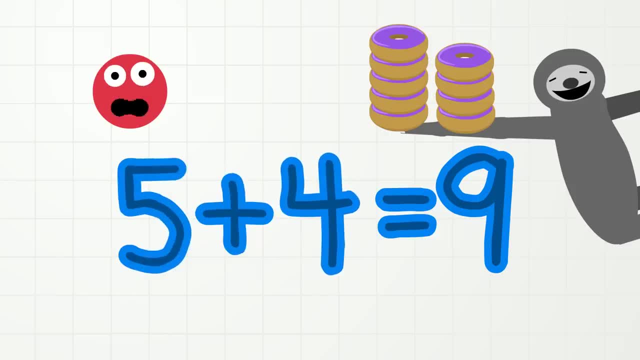 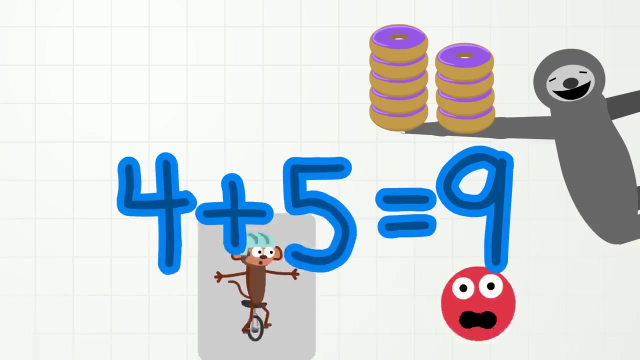 9, and 5 plus 4 also equals 9.. 4 plus 5 equals 9, and 5 plus 4 equals 9.. Everybody: 4 plus 5 equals 9, and 5 plus 4 equals 9.. Happy sloth: 4 plus 5 equals 9, and 5 plus 4 equals 9.. 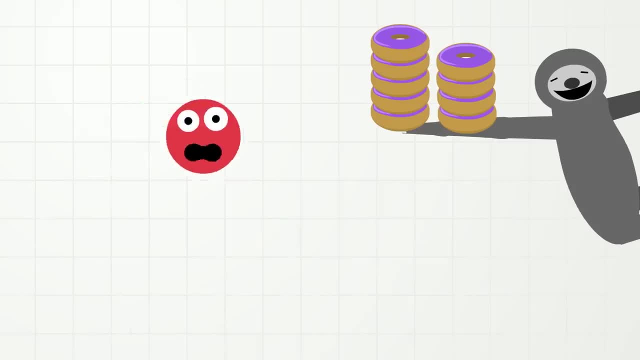 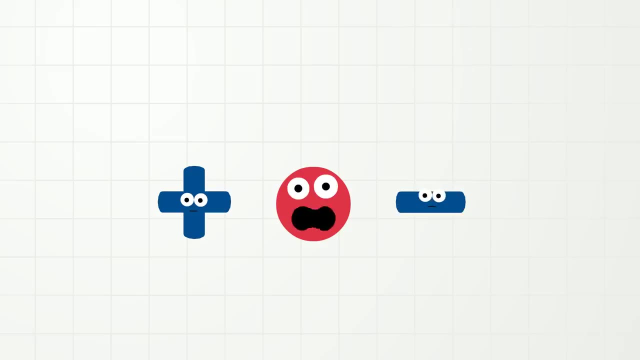 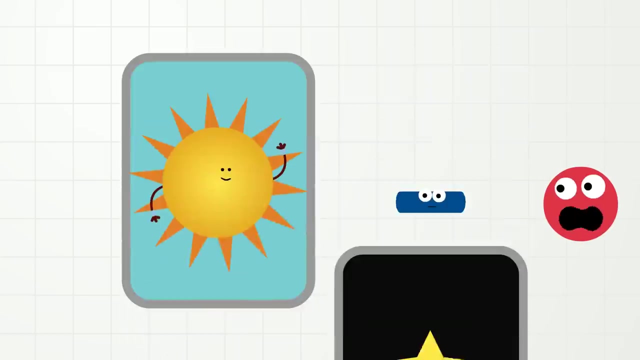 Okay, that's enough. Hey wanna know something? Of course you do. The plus sign and the minus sign are kind of like opposites. You know opposites, Just like happy and sad, big and small, and daytime and nighttime, Opposites, Opposites. 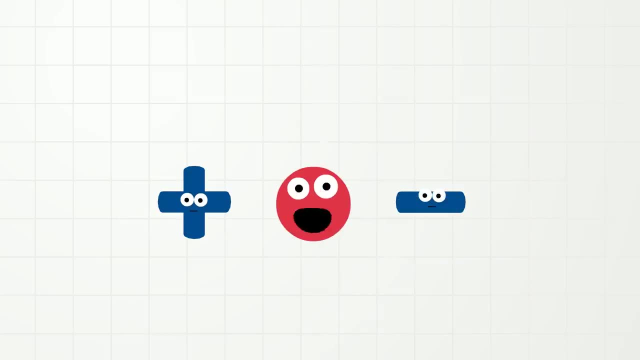 And we can use the plus sign and the minus sign in opposite ways, with the same numbers, to check if our math is correct. No, really watch. If 5 plus 4 is equal to 9, then 9 minus 4 is equal to 5.. Same numbers, different order and different signs, but both are correct. 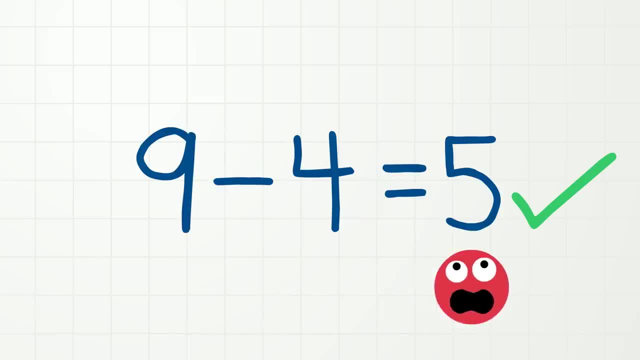 5 plus 4: equals 9.. Correct 9 minus 4: equals 5.. Correct 5 plus 4: equals 9.. Correct 9 minus 4: equals 5.. Correct 5 plus 4: equals 9.. 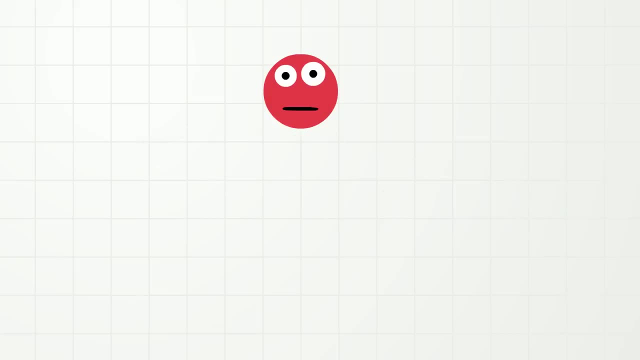 Correct: 9 minus 4 equals 5.. Correct. Okay, that's enough. Okay, let's do one last example of adding, but with some different numbers and different doughnuts: Whoa, sprinkles, Wow. So this one may be a little tricky. We have 1,, 2,. 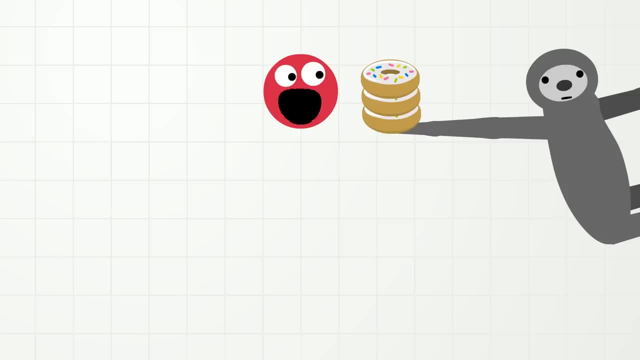 3 doughnuts and we add no more doughnuts. So now we have anybody know That's right: 3 doughnuts. Do you know what is the number we use when we don't have anything? That's right: 0!. 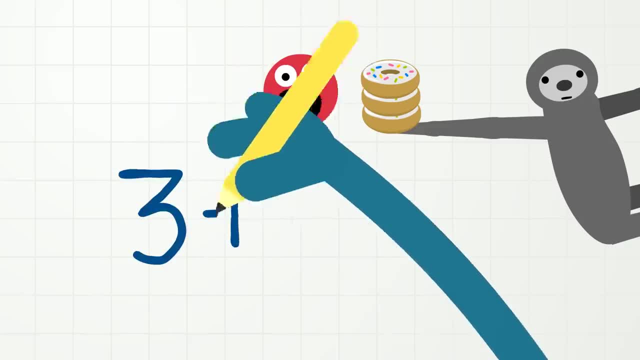 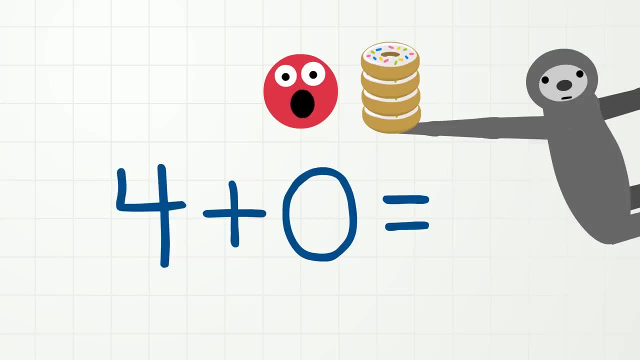 0!. Yeah, So that means 3 plus 0 equals 3.. And what if we had 4 doughnuts and we added 0? That's right, 4. Plus zero equals four. And so even if you had a really really, really high number of doughnuts, like 17,, and added 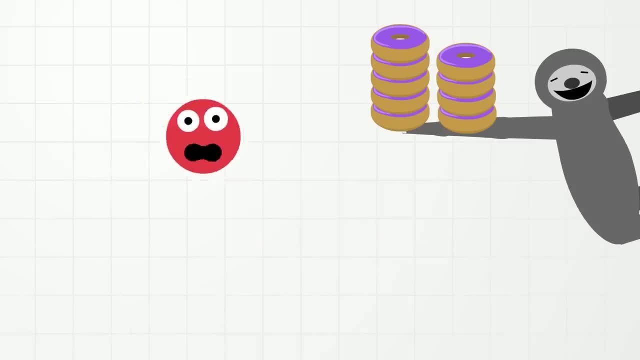 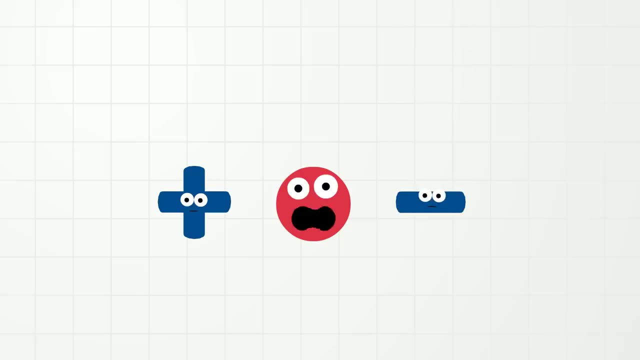 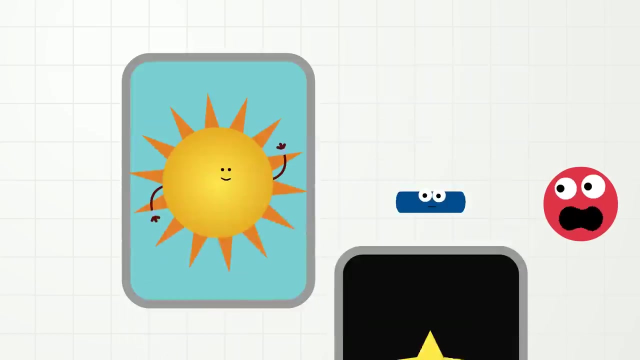 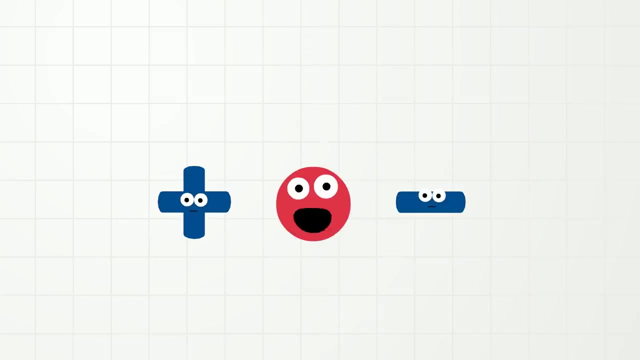 Okay, that's enough! Hey, wanna know something? Of course you do! The plus sign and the minus sign are kind of like opposites. You know, opposites. Just like happy and sad, big and small, and daytime and nighttime. Opposites! Opposites! And we can use the plus sign and the minus sign in opposite ways with the same numbers to check if our math is correct. No, really, watch! If 5 plus 4 is equal to 9, then 9 minus 4 is equal to 5. Same numbers, different order, and different signs, but both are correct! 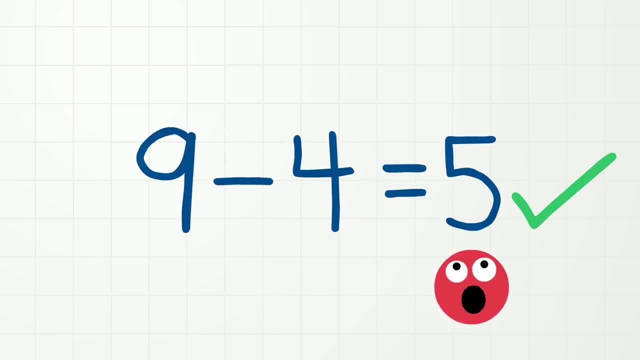 5 plus 4 equals 9. Correct! 9 minus 4 equals 5. Correct! 5 plus 4 equals 9. Correct! 9 minus 4 equals 5. Correct! 5 plus 4 equals 9. Correct! 9 minus 4 equals 5. Correct! Okay, that's enough! 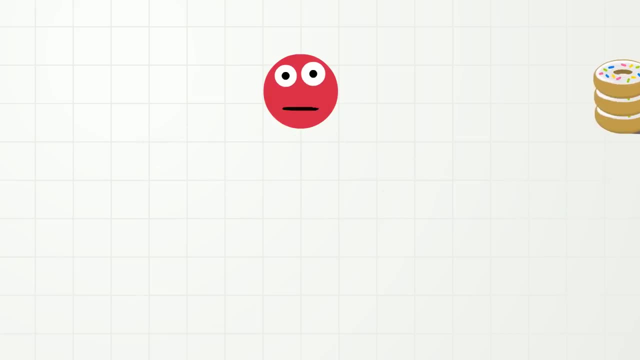 Okay, let's do one last example of adding, but with some different numbers and different doughnuts. 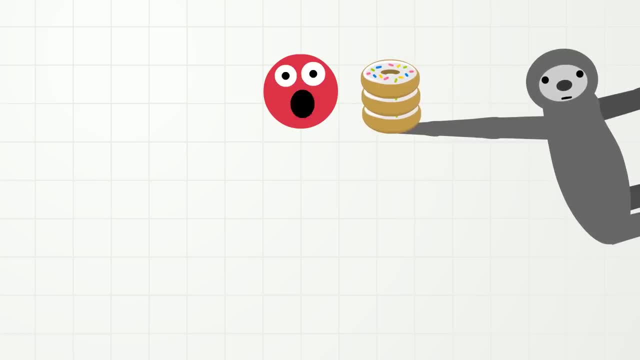 Oh, sprinkles! Wow! 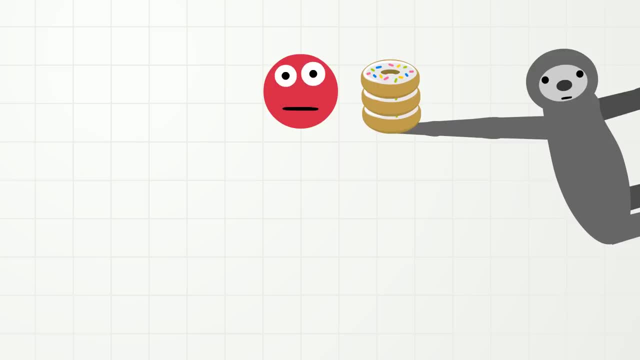 So, this one may be a little tricky. We have 1, 2, 3 doughnuts, and we add, uh, no more doughnuts. So now we have, anybody know? That's right! 3 doughnuts! 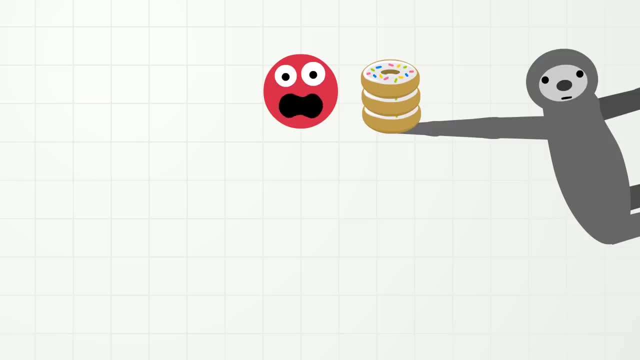 Do you know what is the number we use when we don't have anything? That's right! Zero! Zero! Yeah! 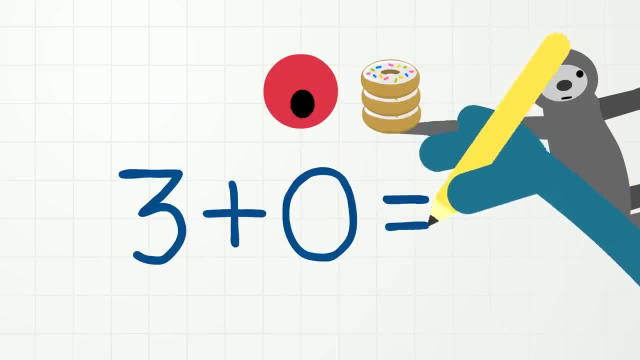 So that means 3 plus 0 equals 3! 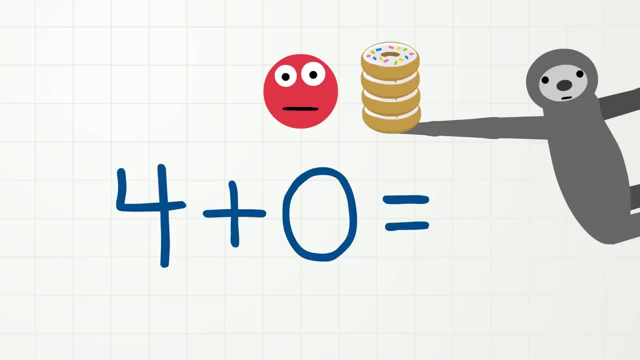 And what if we had 4 doughnuts and we added 0? That's right! 4 plus 0 equals 4! 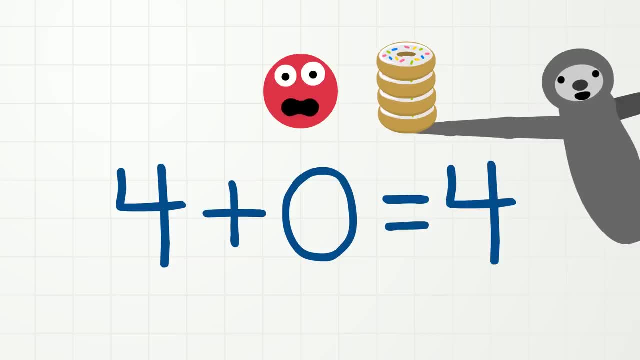 And so even if you had a really, really, really high number of doughnuts, like 17, and added 0, you would still have 17 doughnuts! Yay!